usually you don't know of people going around donating bone And, in fact, usually you don't know of people going around donating bone. And, in fact, usually you don't know of people going around donating bone And, in fact, usually you don't know of people going around donating bone. 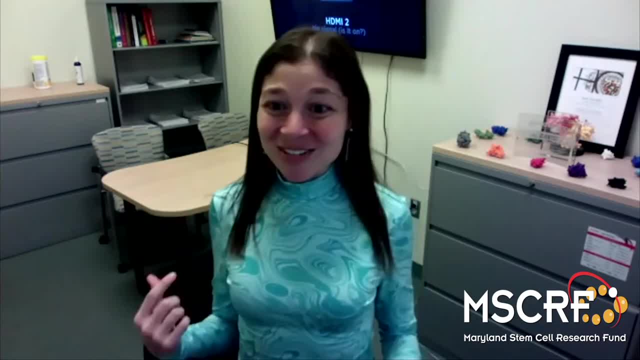 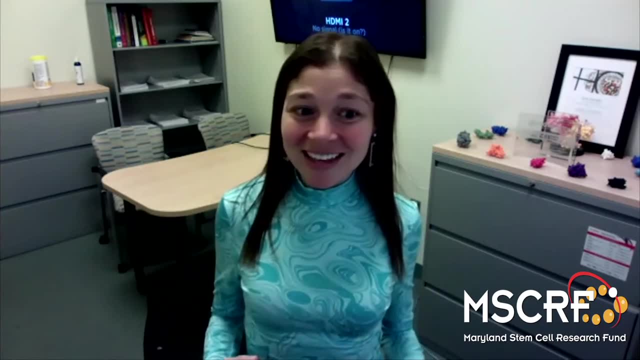 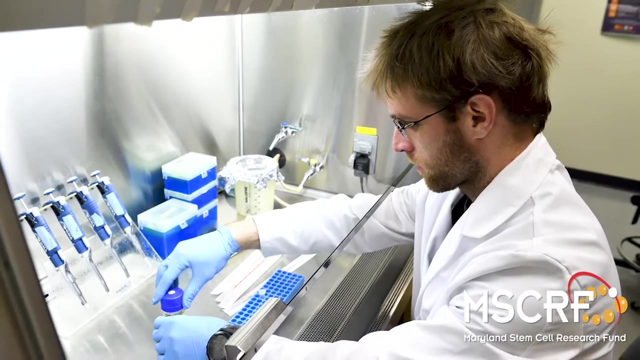 The bone grafting procedure comes from one part of your body to another, and that can cause a lot of complications. First of all, there's risk of infection and risk of damage at the site of the grafting. In addition, it's very costly procedure and also the limited supply. And so what people? 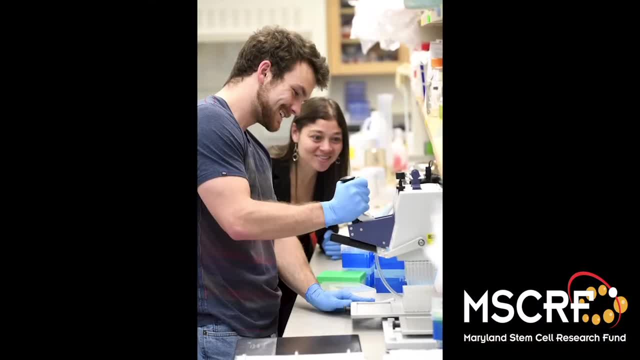 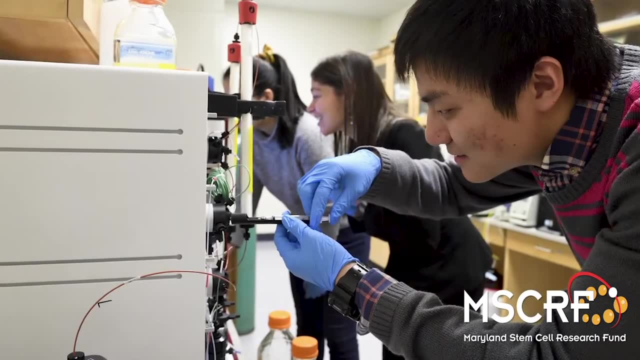 have come up with as an alternative is what's called tissue engineering. What it entails is basically taking a biomaterial scaffold and loading that up and then taking it to the balcine, And typically, when we take it in the breecus, if you're LA, we take it to the 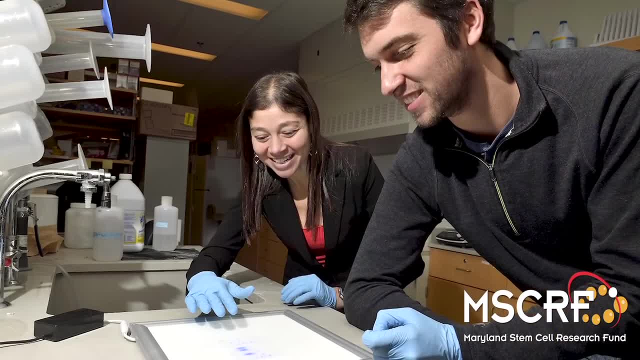 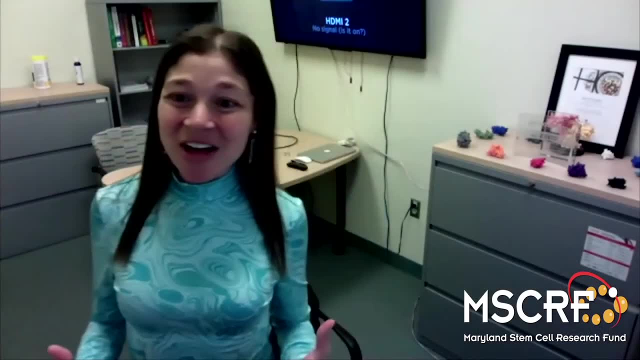 bronchial wall and then we take it there Once we're trying to re-train that, we just pass that trailers from injury and that's that imagine being merely a chapter in the cycle of the colorectal lung or whatever, of the Phantom's blood which is the lives of the curative. 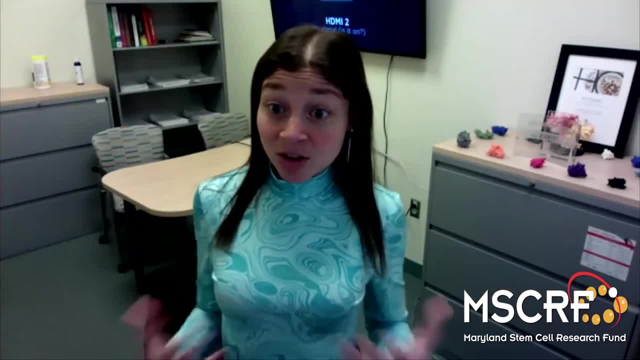 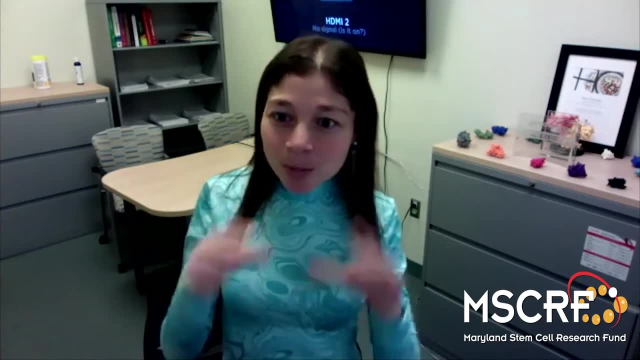 part of the process. Also, we can't do some training undergraduates on how to doige somatic surgery, because if you do it in the retina it takes some time for the tomography to Mantra, because the pancreatic longace episode of Women'schen is done in the eggs, which is a truly 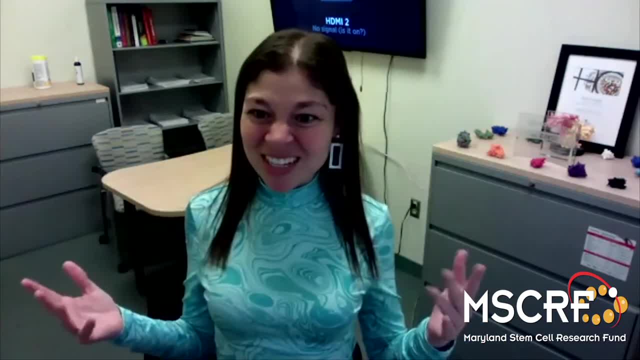 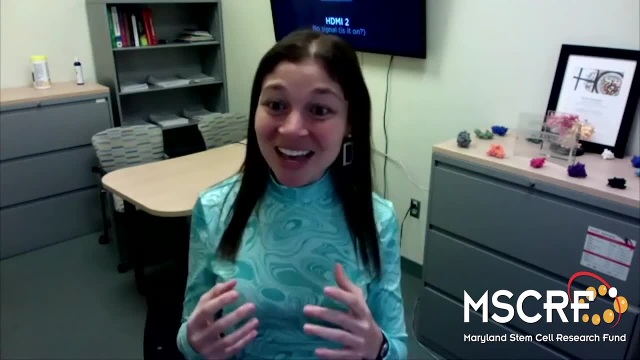 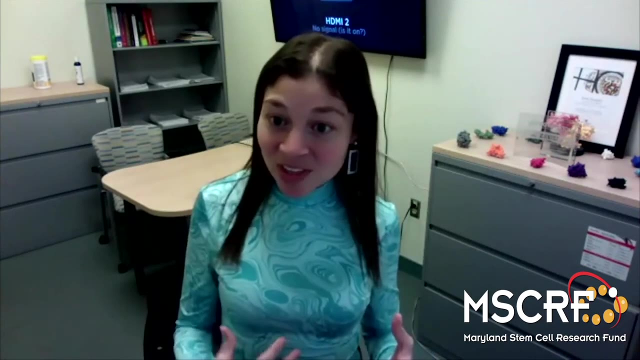 body, but they also stimulate the cells all over your body, which can lead to cancer and other complications, And so our idea as protein engineers and protein designers, was to actually create these designer proteins that would only interact with the scaffold that you put into somebody's body. 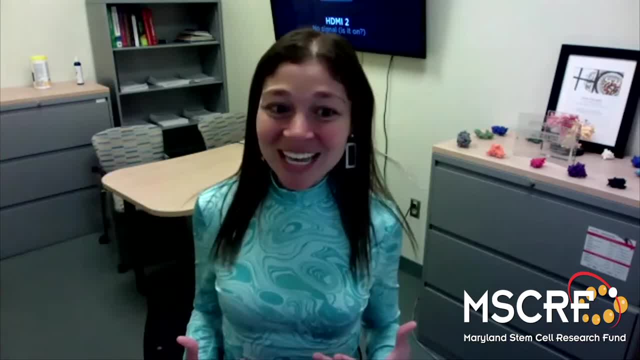 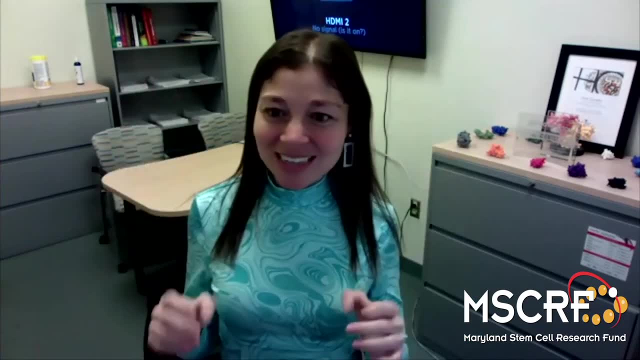 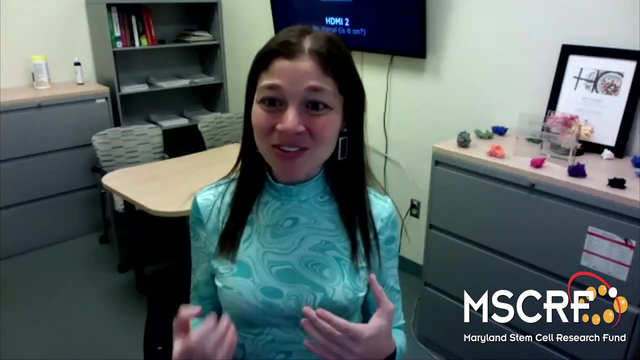 and not interact with any other cells in your body, And the idea there was that by creating these what we call orthogonal protein systems, or basically fake proteins, we can actually create something that would very specifically and safely be able to stimulate bone growth in a human being and be a clinically translationally 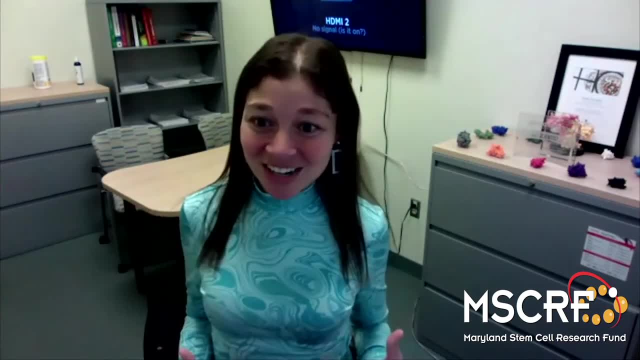 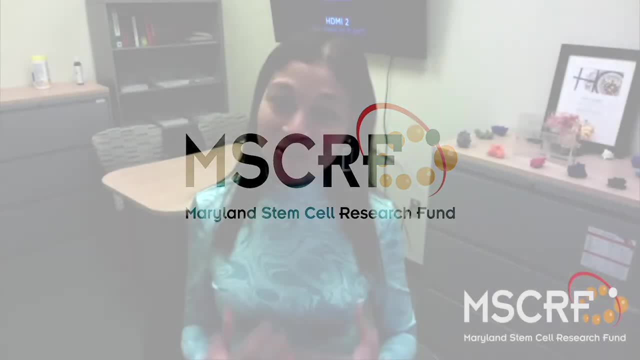 relevant application of tissue engineering technology. We really appreciate that Maryland Stem Cell Research Fund has supported this work And this was actually one of my first research grants as a starting principal investigator here at Johns Hopkins And I was really excited to be part of that.